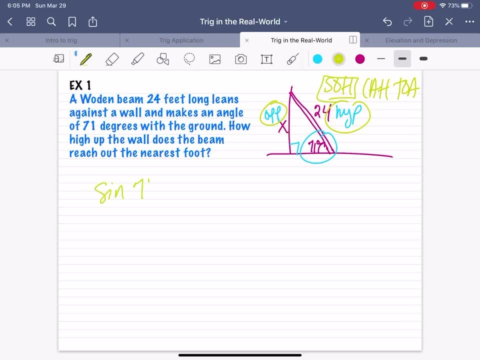 use sine. So the sine of 71 degrees is equal to opposite, which is x, over the hypotenuse, which is 24.. So you already know how to do this part. The only new part is the word problem. So you multiply both sides by 24. 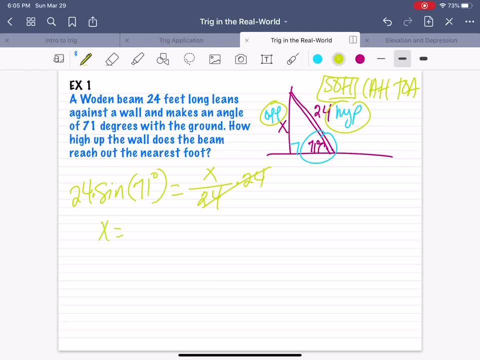 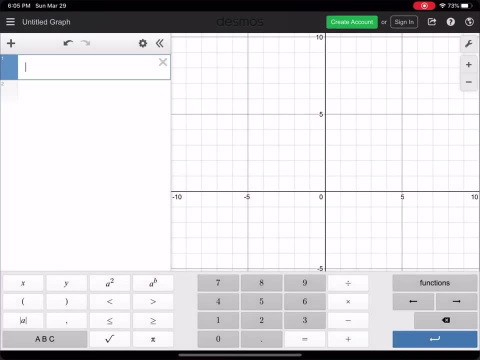 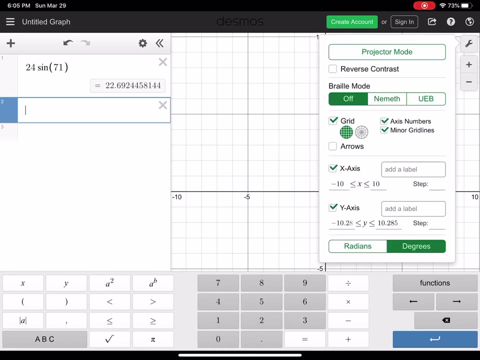 and x is equal to 24 times the sine of 71 degrees. So let's go to Desmos calculator: 24 times the sine of 71 degrees. Let me make sure my calculator is in degrees And it is, So it is 22.7.. 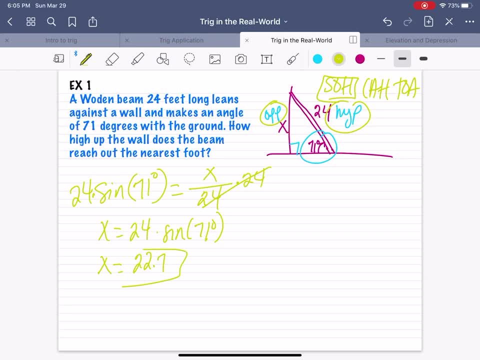 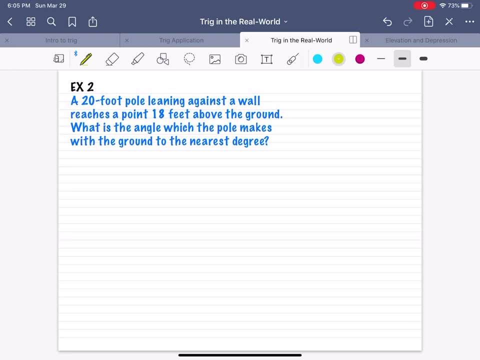 So the value of x is 22.7.. Example two: a 20 foot pole leaning against the wall reaches a point 18 feet above the ground. What is the angle at which the pole makes with the ground to the nearest degree? So again we have a wall. 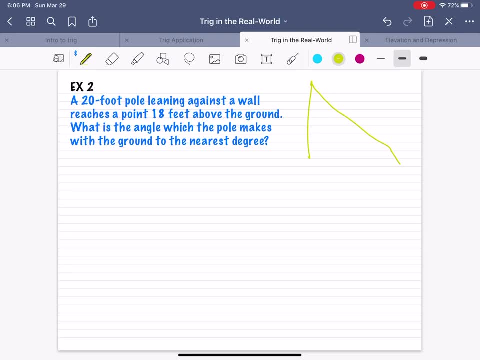 and then there is a pole leaning on that wall. we have a wall and a pole, a 20-foot pole. so the pole is 20 feet long and that pole reaches 18 feet above the ground. so here's the pole, here's the ground. this right here is 18 feet question. 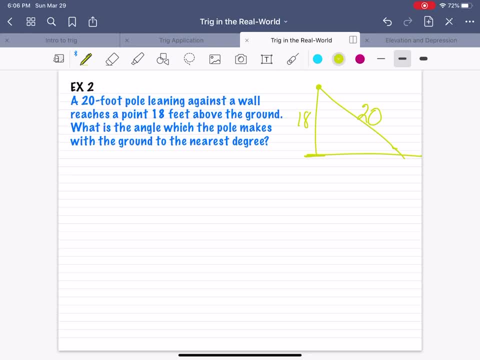 what is the angle at which the pole makes with the ground? here's the ground, here's the pole. it's asking for this theta, so let's label our picture using this theta. this right here is the opposite, right across from it, and this is the hypotenuse right across the 90 degree angle. so, of course, 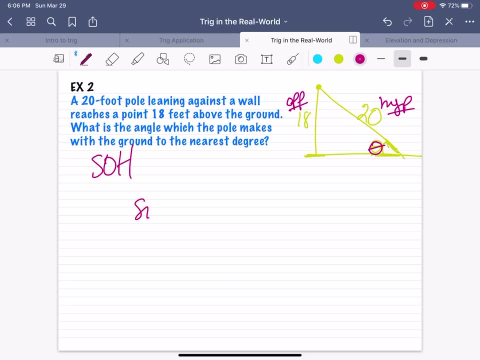 we're going to use so again from sohcatoa. so the sine of theta is equal to opposite over the hypotenuse and that's going to help you solve for theta. so to get the theta by, so you have to get rid of the sine. 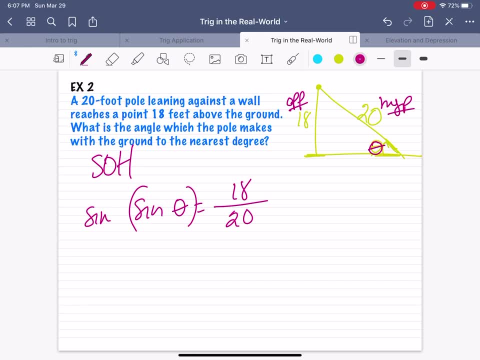 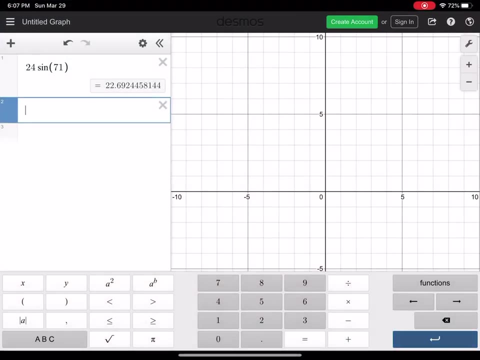 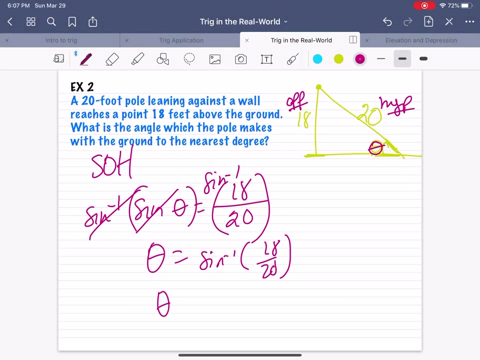 so you do the inverse sine of both sides and you go straight to desmos calculator. inverse sine of 18 over 20. inverse sine of 18 over 20: 64.2. so theta, the angle that the pole makes with the ground, it is 64.2 degrees. 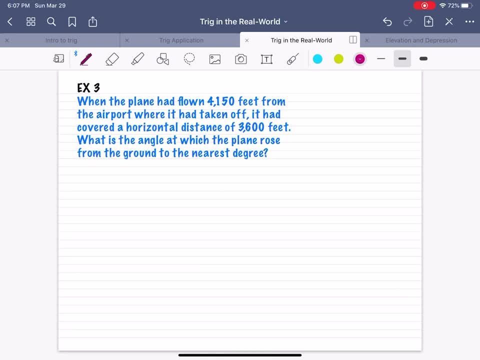 example three: when the plane had flown 4150 feet from the airport where it had taken off, it had covered a horizontal distance of 3600 feet. what is the angle at which the plane rose from the ground to the nearest degree? okay, so let's draw a triangle. so let's draw a triangle. here's the 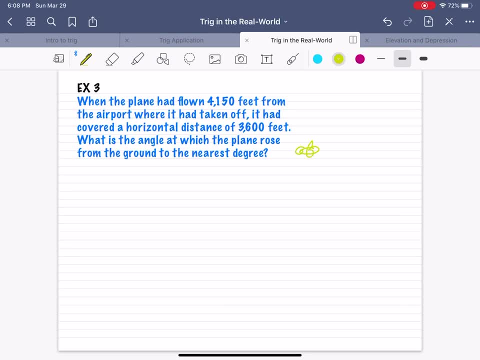 let's say, our plane starts here on the ground. here's the ground the plane takes off and here's the altitude, how high off the ground the plane is. so when the plane had flown, 4 150 feet from the airport, which means- or how pine news is- 4150 covered a horizontal distance. so this right here. 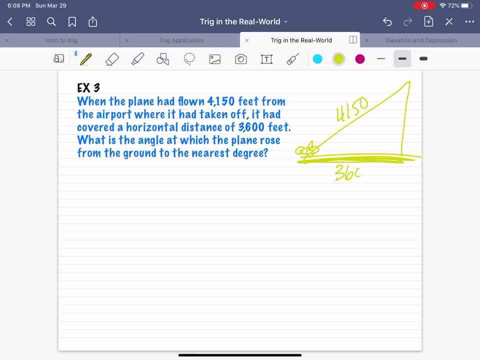 is horizontal distance, so that right there is 3 600 feet. the question is: what is the angle at which the airplane rose from the ground to the nearest degree, so that right there is the theta? so we have our triangle. let's label the picture. this is the adjacent, this is the hypotenuse. 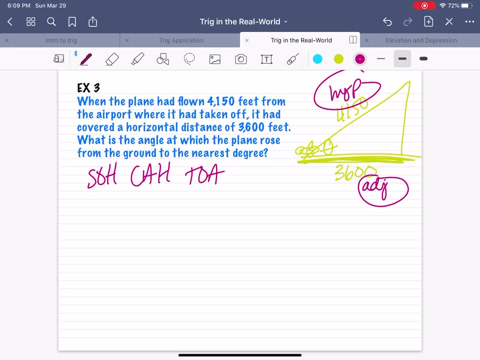 since we have adjacent and hypotenuse, we're going to use cosine. so the cosine of theta is equal to the adjacent over the hypotenuse and that's going to help us solve for cosine to get rid of the cosine. you do inverse cosine on both sides. 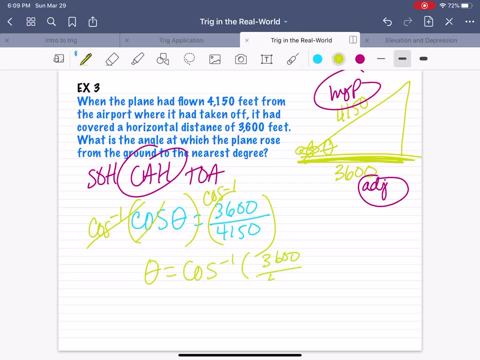 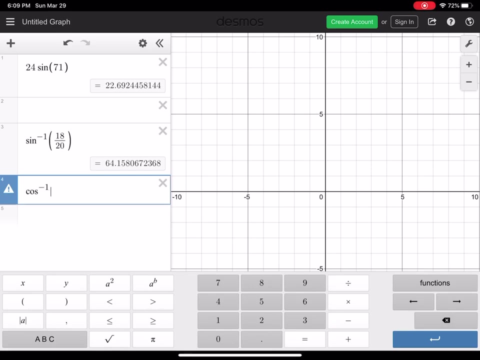 theta equals inverse cosine of 3600 over 4150.. so it does most calculator inverse cosine of 3600 divided by 4150.. what we have to do now Let's see how we can estimate thejet's velocity by focusing on the part of the angle where it's 29 degrees. 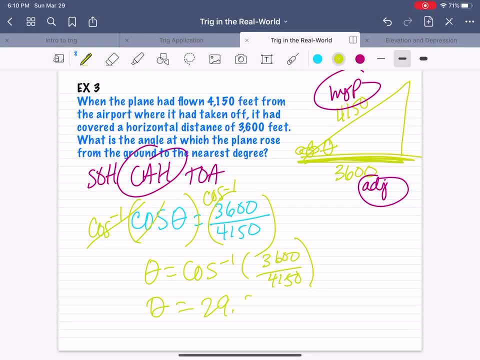 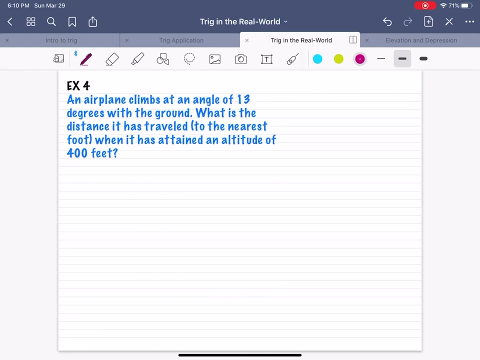 and trying to set that into the最高. these are the dirts one. here's the Fast todos here from the FD n Schrodinger. those forces are are really touchscreen set for形状. get this into the nearest degree. it is 29.8. age set to the nearest degree. this right here is bigger than five, so let's say 30 degrees. so the angle here will be 30 degrees. example 4: engineering. the plane climbs at the angle of 13 degrees with the ground. what is the distance it has to land? at an angle oficane, because the ground is slice, the Nabak' es, while it is a lot smaller than where you know什么. 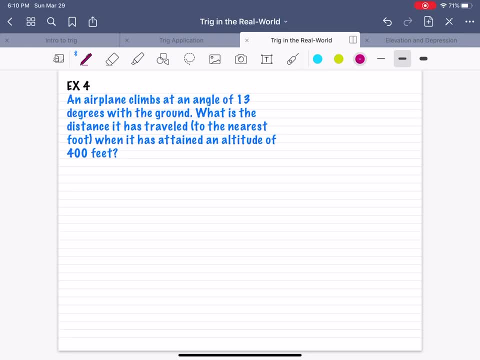 it has traveled to the nearest foot when has attained an altitude of 400 feet. so we draw the picture: airplane starts right here, climbs at an angle of 13 degrees, and meaning this right here is 13 degrees. what is the distance that has traveled? so it'll be the hypotenuse because the airplane starts here. it 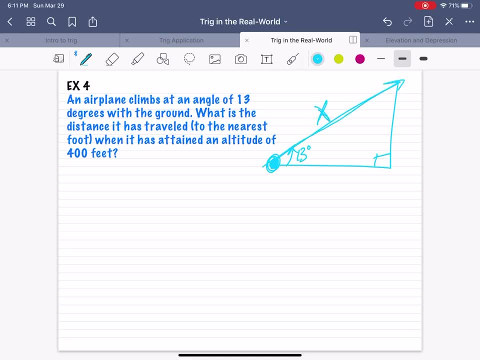 travels this way. so that's the distance it has traveled when the altitude is 400 feet. so remember, altitude is height. so here's your height. this is 400 feet, so let's label the picture using this angle. this side is the opposite and this is the hypotenuse. if you soak a toy, you're gonna use so. so that is the sine of 13. 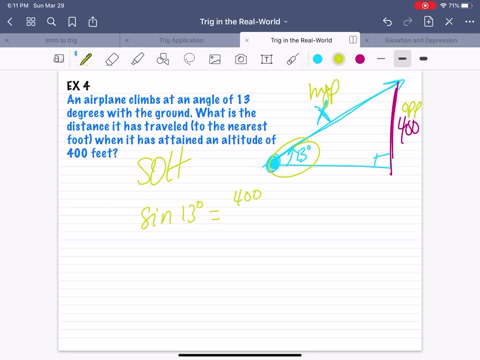 degrees is equal to opposite over hypotenuse. so to solve for X, multiply both sides by X, so you have X times the sine of 13. degrees equals 400. to get the X by itself, you divide both sides by sine of 13 and X is equal to 400 over sine of 13.